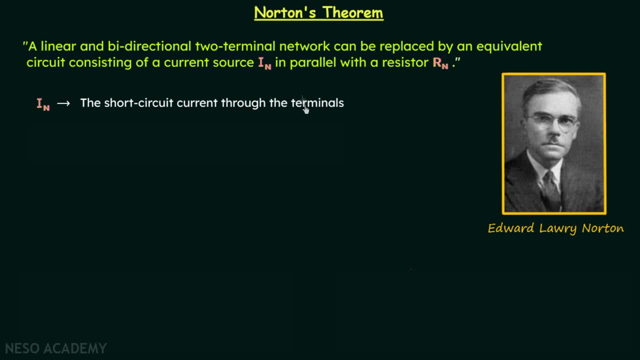 is the short circuit current through the terminals, And when you compare I n with V th, you will find there, in case of Thevenin's theorem, while calculating V th we were open circuiting the terminals and then finding out the voltage across the open terminals known as V th. But 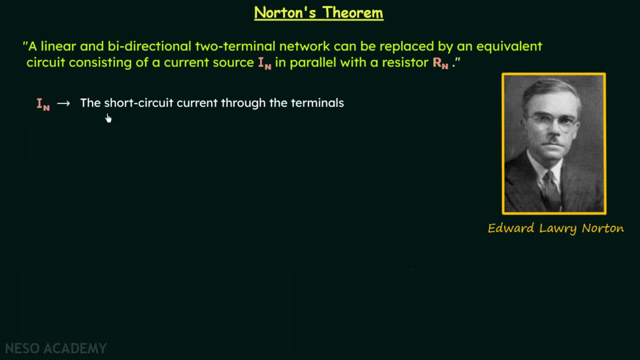 here. in this case, we are short circuiting the terminals and then finding the current, known as I n. This will be more clear after taking one example problem. Now, moving on to Rn, it is the input or equivalent resistance at the terminals when the independent 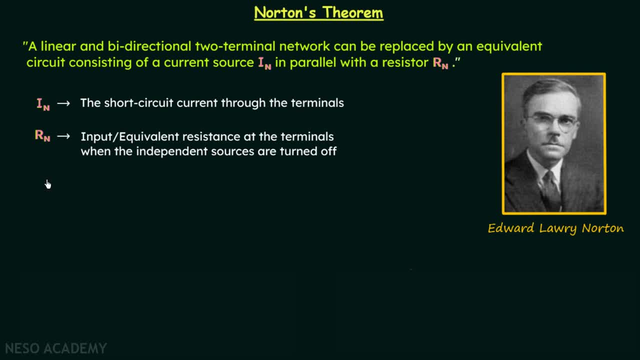 sources are turned off. When you compare this with Rth, you will find they are absolutely equal. So there is no difference between Rn and Rth. We can say that Rn is equal to Rth, So the Norton's equivalent resistance is equal to the Thevenin's equivalent resistance. 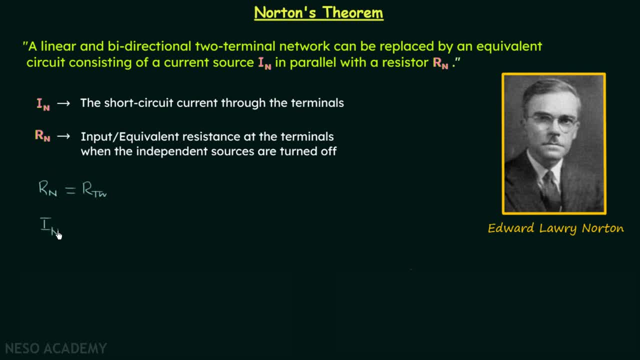 And this current, which is the Norton's equivalent current. it is equal to the Thevenin's equivalent voltage, Vth, divided by the Thevenin's equivalent resistance, Rth, Or we can say that Rth. it is equal to Vth over current Rth. 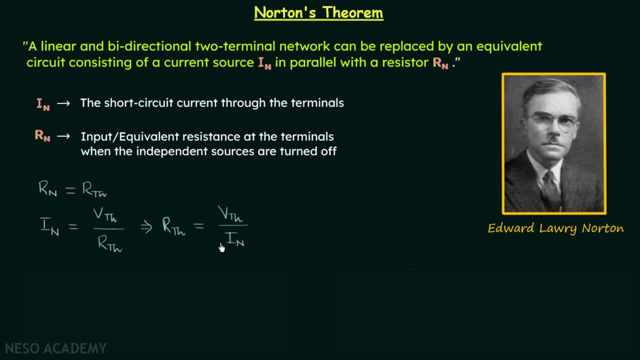 And from this we can say that Rth is equal to Rn and they are equal to Vth over In. And this obtained result here is an important result and we call this source transformation. If you remember, In chapter one of this subject I said we are going to have discussion on source transformation. 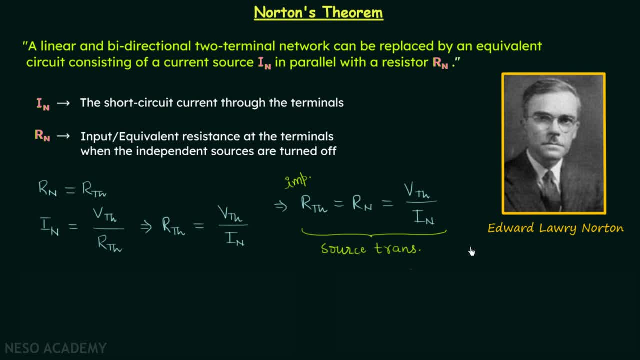 in the fourth chapter, that is, the network theorems chapter, And I said that because source transformation is nothing but Thevenin-Norton transformation. We call it Thevenin-Norton transformation And this is one very important topic And therefore we will have discussion on this particular concept in the next presentation. 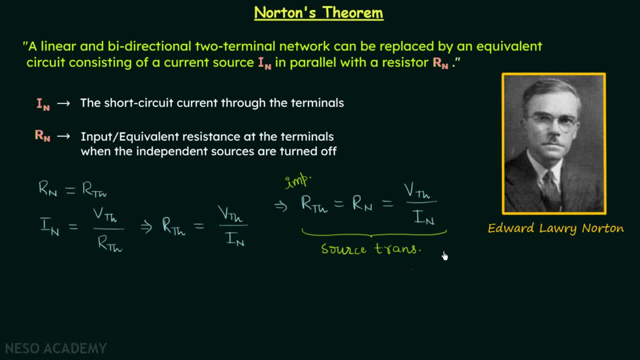 and we will solve some questions Which will help us understand the application of source transformation in a better way. Now, moving on to the next point, in which we will understand what has to be done with the independent and the dependent sources in case of Norton's theorem. 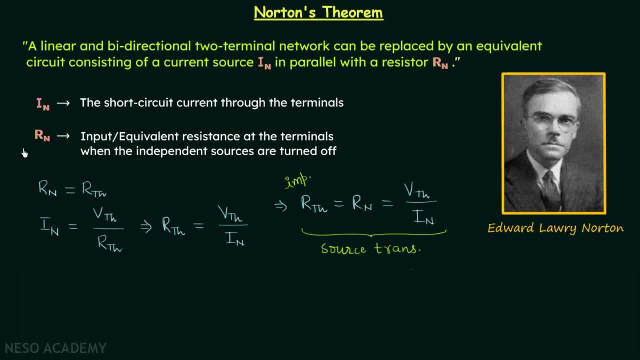 While calculating Rn, we turn off the independent sources, but we leave the dependent sources as they are, And therefore we can say that the independent and the dependent sources are treated the same way as in Thevenin. Now to summarize the Norton's theorem, I have taken this diagram: 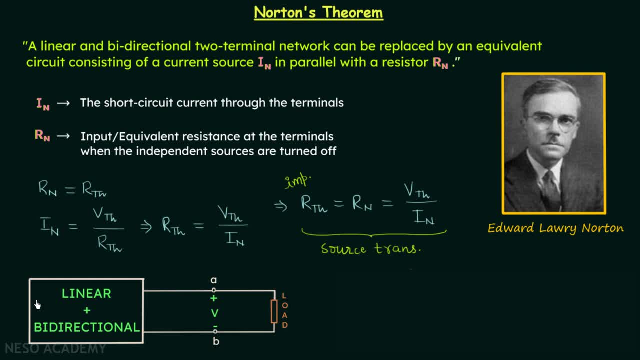 This black box is representing a complex, linear, bidirectional, two-terminal network, And across this network a load is connected and this load is changing. So to minimize our calculations, we will replace this complex network by In, connected in parallel with Rn, And this is our Norton's equivalent circuit. 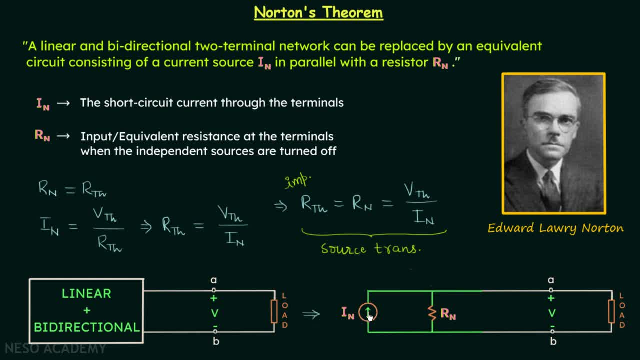 So we are replacing this network by In, connected with Rn in parallel, and we are getting an equivalent network and we will perform the analysis on this network instead of this network. So this is all for the introduction. Now we will move on to one example problem. 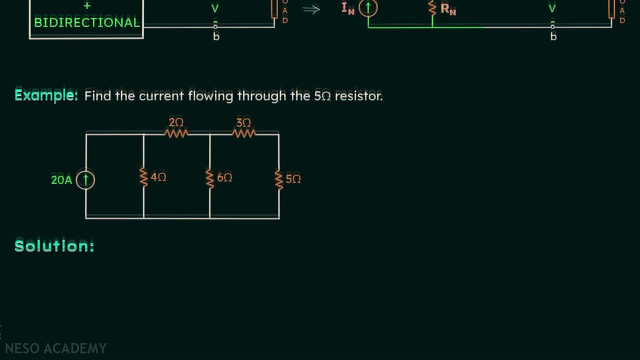 And with the help of this problem we will try to understand how to calculate In and Rn and then have the Norton's equivalent circuit. So this is our question and according to the question, we are required to find the current flowing through the 5-ohm resistor. 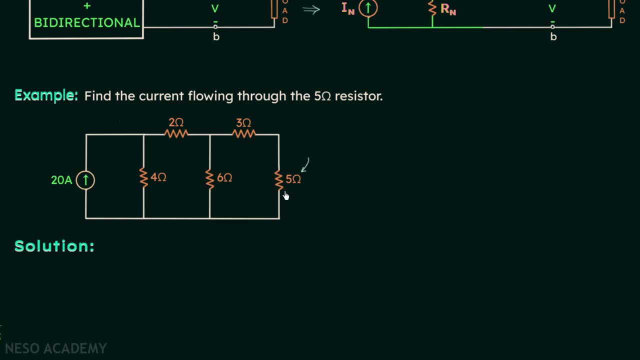 When you observe the given network, you will find this is 5-ohm resistor and we need to find the current through this resistor. So let us try to understand how to find current with the help of Norton's theorem. We will first calculate current In and then we will calculate Rn and finally we will have 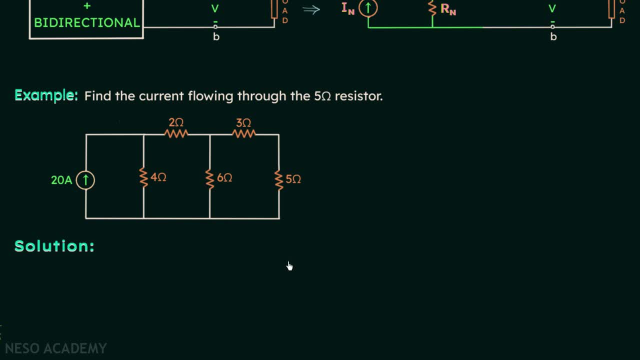 the Norton's equivalent circuit. So let us move on to the calculation of In. and for that, we are required to make one change in our network. We will short circuit the load like this, and then we will assign the Norton current In like this. Now, here we are, following one convention which you must understand. 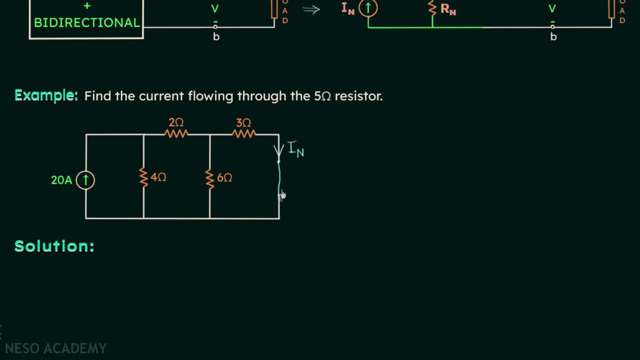 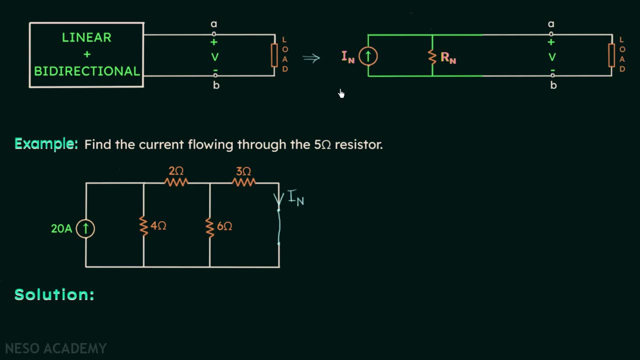 You can see the direction of current In It is downward. And when you have Your Norton's equivalent circuit, this one, the direction of In this current should be upward. Now understand why we are taking the directions as mentioned. Focus on the load branch in the two cases. 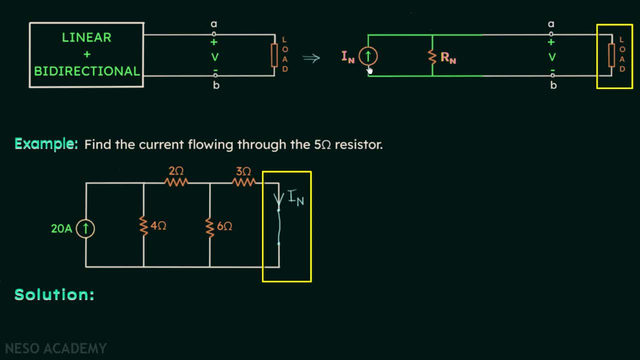 In the case number one, while calculating In, we are having the direction downward in the load branch. And in case number two, while having the Norton's equivalent circuit, the direction of In is upward, So that the direction of current through the load branch is downward. 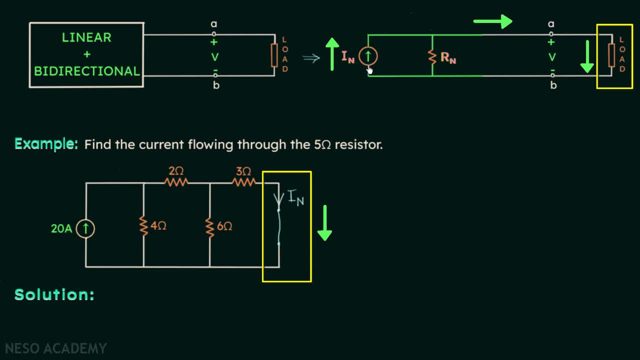 This means we are trying to have the same direction of current through the load branch. So remember, while calculating In, take the direction downward and in Norton's equivalent circuit, take the direction upward. and vice versa can also be done. That means, while calculating In, take the direction upward and in Norton's equivalent, 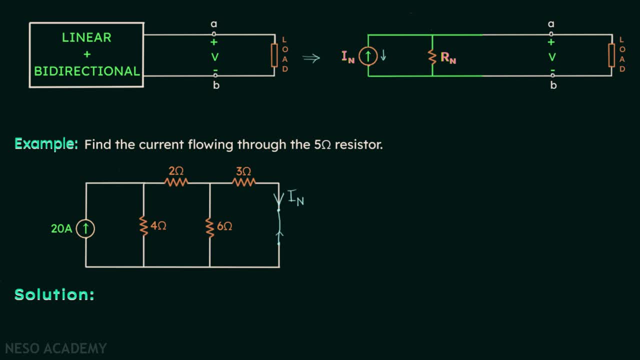 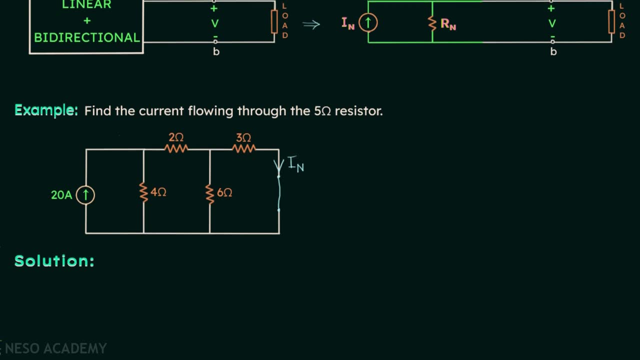 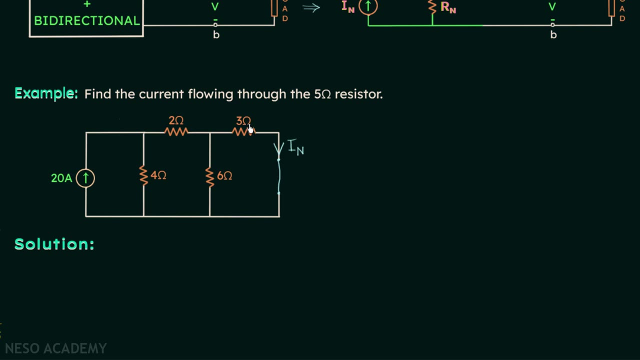 circuit. So the direction downward, But I will follow this convention. So in this way we have our network ready to calculate current In. When you focus on these two resistors, you will find they are in parallel, So their equivalent will be equal to 2 ohms, and then that 2 ohms will come in series with 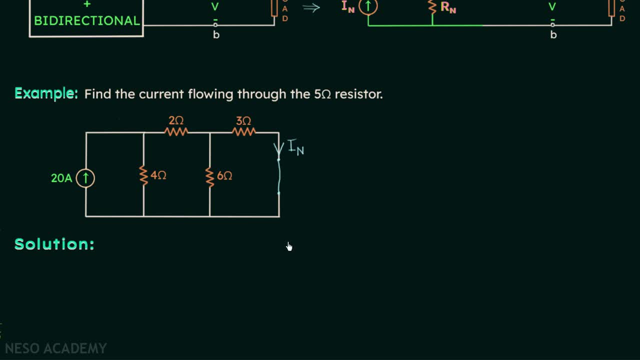 these 2 ohms, So we have 4 ohms equivalent resistance for this particular section of the network And therefore we have 4 ohms equivalent resistance for this particular section of the network And therefore we finally have 4 ohms connected in parallel with 4 ohms. 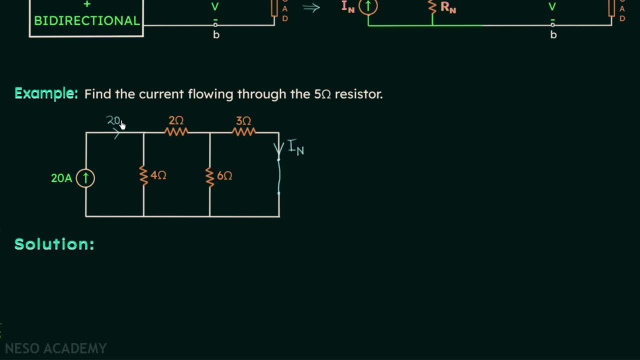 And this 20 amperes of current at this node will have two paths. The first path is offering 4 ohms of resistance and the second path is also offering the 4 ohms of resistance, So the current will get divided equally. 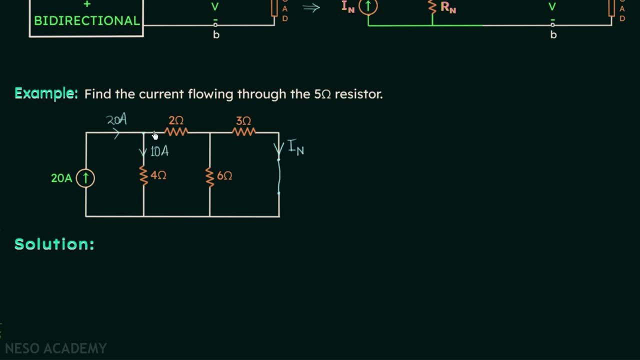 In this branch, it will be 10 amperes. In this branch, it will be 10 amperes. In this node, it will be 10 amperes. In this node, it will be 10 amperes. In this node, it will be 10 amperes. 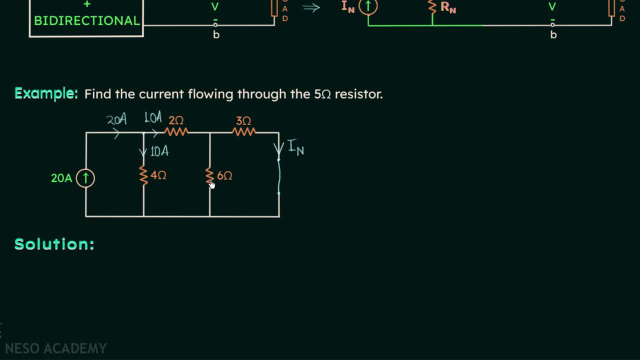 and in this branch it will be 10 amperes. Now this 10 amperes current at this node will have two paths, so it is getting divided and therefore we can use the current divider rule to find out IN: IN it will be equal to the total current entering the node, which is 10 amperes multiplied. 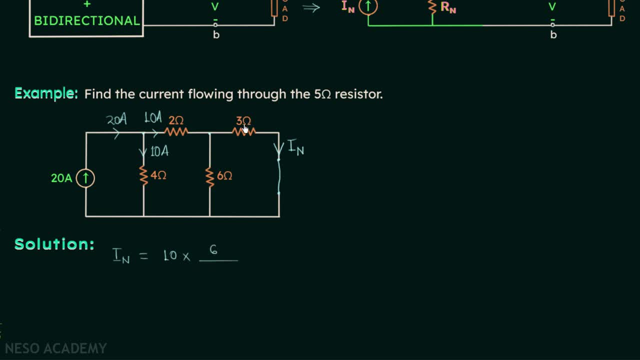 to the other resistance divided by the sum of resistance values. From here we will have current IN the Norton's equivalent current equal to 20 over 3 amperes. So we are done with calculating Norton's equivalent current. Now we will move on to the calculation of Norton's. 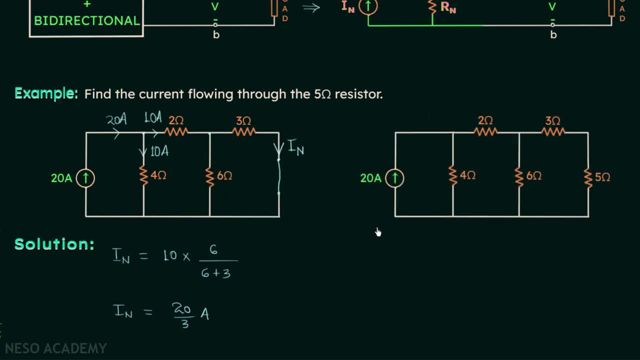 equivalent resistance, And for this we are required to make two changes in our network. The change number one is open subnet. The change number two is turning off the independent sources present in the network. There is only one independent source and it is a current source, So to turn it off we will replace. 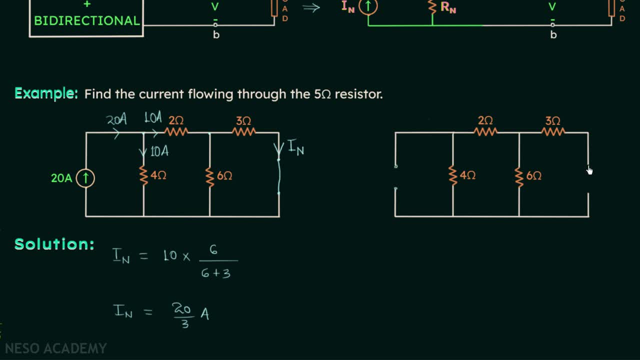 it with an open circuit And we know Rn is nothing but Rth, So it is the resistance when looked from these two terminals. in this way, Now to find out Rn, we will observe the combinations we have here. Four is in series with two. 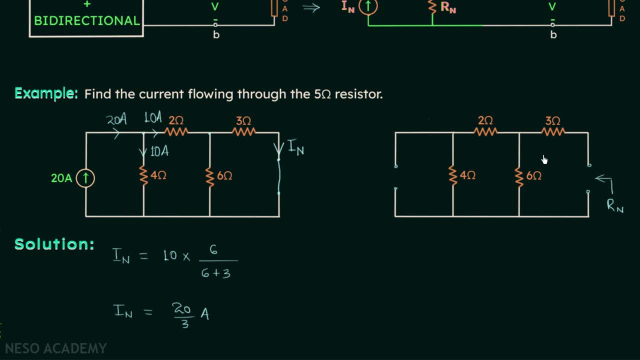 then they are in parallel with six, and then this combination is in series with three, So Rn it will be equal to 4 plus 2.. Then they are in parallel with 6.. And then this combination is in series with 3.. So plus 3.. 4 plus 2 is 6.. So we have Rn equal to 6 in. 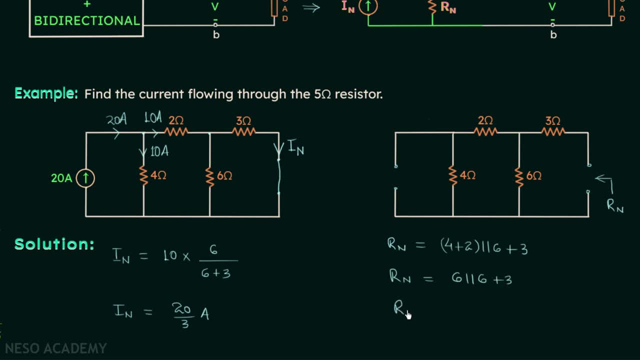 parallel with 6 plus 3.. 6 parallel with 6 is equal to 3. So we have 3 plus 3.. So Rn is equal to 6 ohms, And now we will have our Norton's equivalent circuit. In is connected in parallel with Rn and